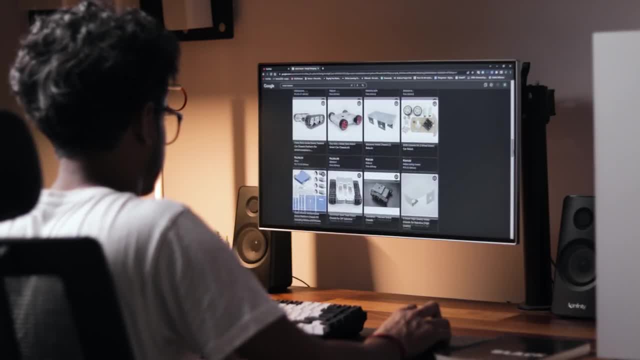 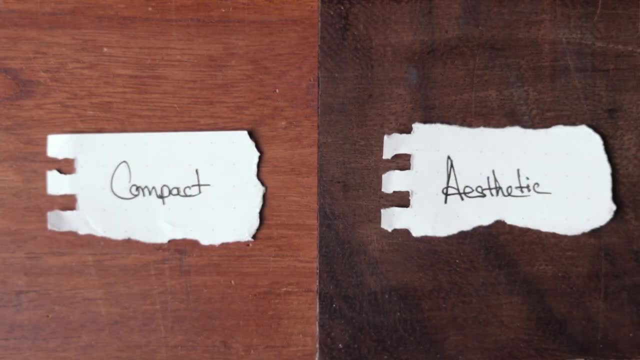 find it online, but unfortunately I couldn't find the specific one that I'm looking for. Sure, there are a few models available, but most of them kinda look same and boring. Well, I want mine to be compact and aesthetically pleasing, So in the end I've decided to. 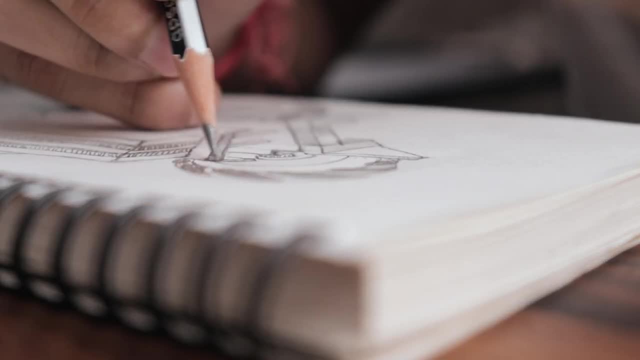 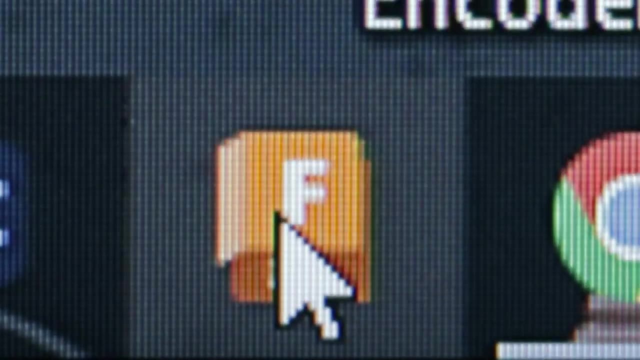 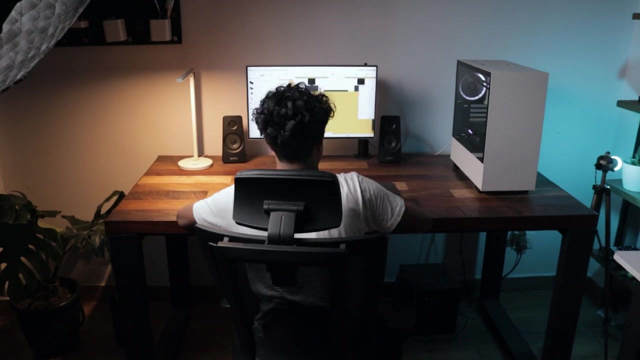 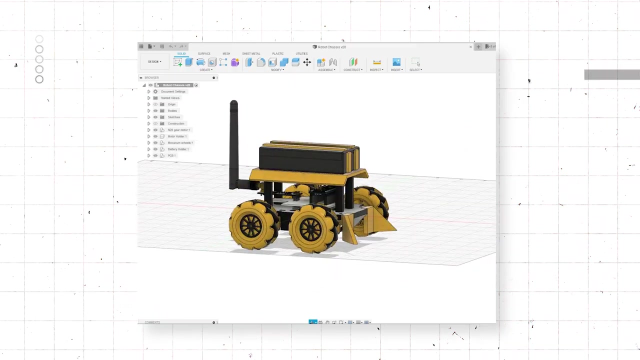 design it by myself. I know I'm not good at drawing, but for reference I think it will get the job done. Alright, it's time to transform this 2D drawing into a 3D model. My design is ready and I'm pretty happy with the result. Now let's fire up the 3D. 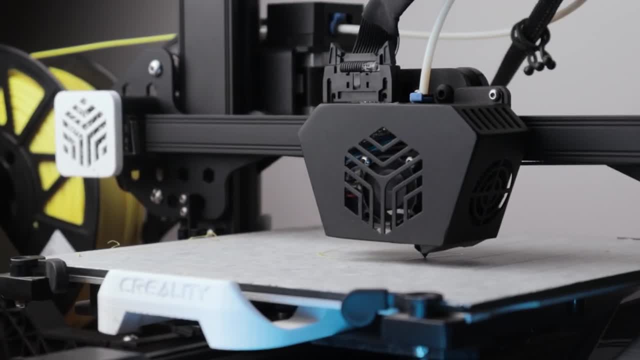 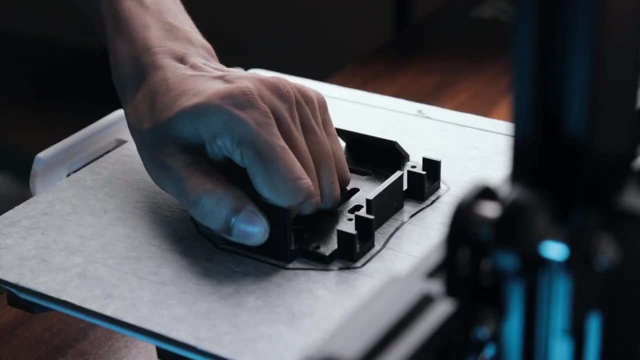 printer and start bringing these parts to life. It's gonna take a while to complete all the parts, so let's fast forward the process a little bit. After 10 hours of continuous printing, the 3D printed parts are now finally ready to be printed. 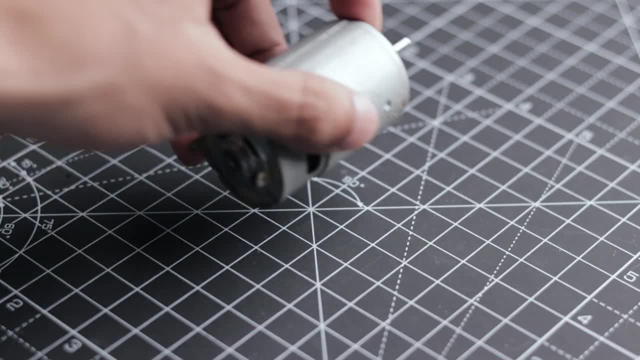 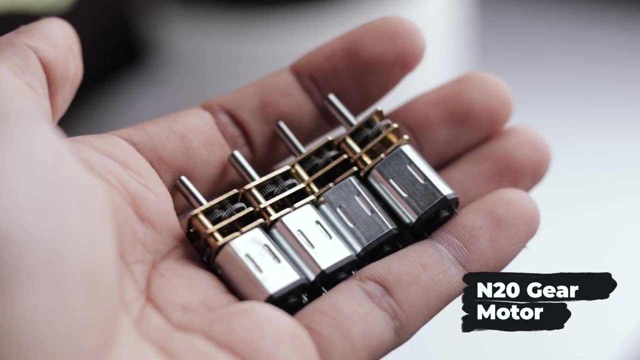 So let's get started Now. it's time to start the assembling part. First, let's start with the motor. Check out these N20 Micro Metal Gear motors. These are exactly what I need for this little project, But before mounting them to the robot chassis first, let's quickly solder wires to each. 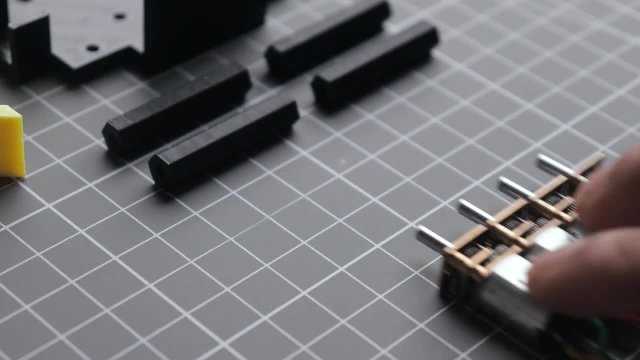 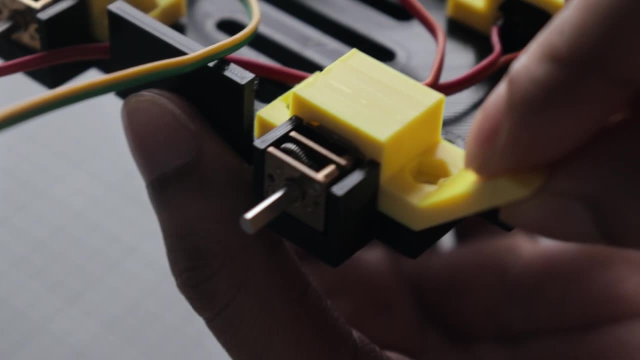 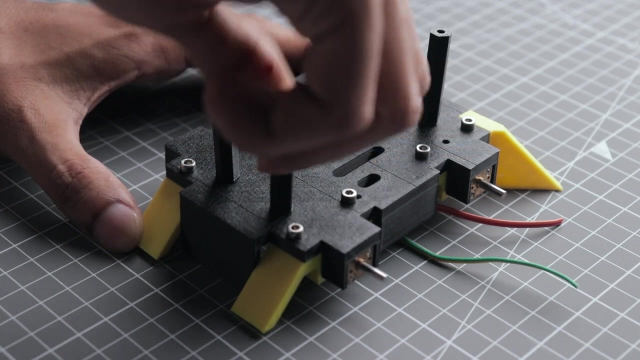 motor connector. With that done, all the motors are good to go. Now let's quickly mount them onto the motor holder and attach the assembly to the robot chassis using some M3 screws. Next, let's mount these 3D printed stand-offs to create enough space for the electronics. 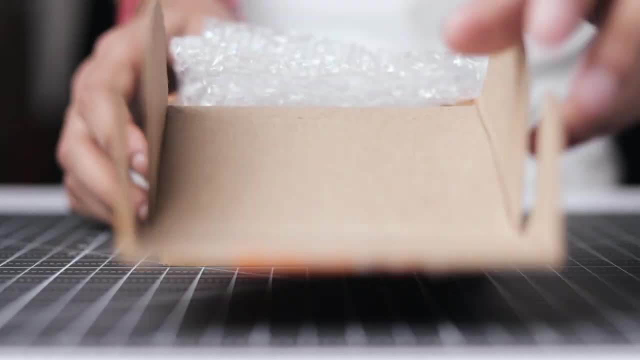 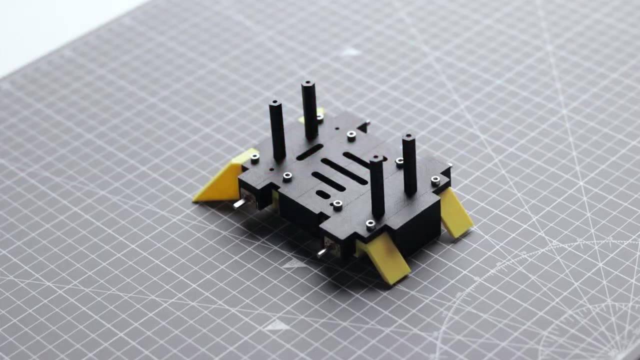 Now, instead of these boring old rubber wheels, I'm using these Mecanum wheels. These wheels will allow this robot to move in any freaking direction you can think of. How cool is that? Okay, time to mount these wheels to the motor shafts, With the robot chassis almost completed. 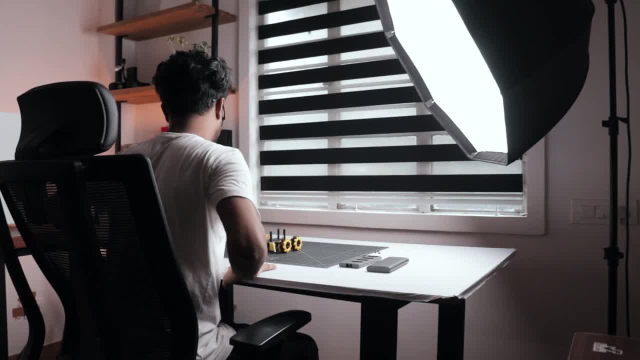 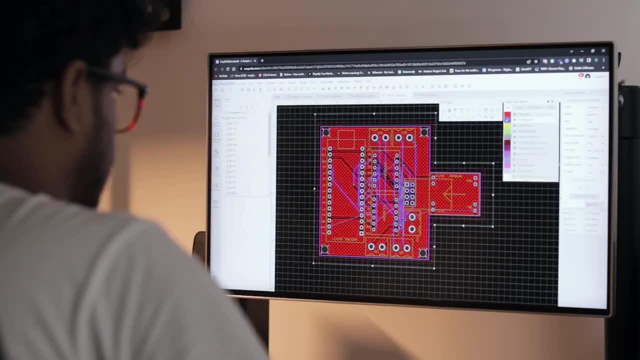 we are ready to move on to the next step. Now it's time to work on the circuit. So I headed back to my desk and started designing the circuit using EasyADA, which is an online circuit design tool. After completing the design, I uploaded the cover files to JLCPCB's. 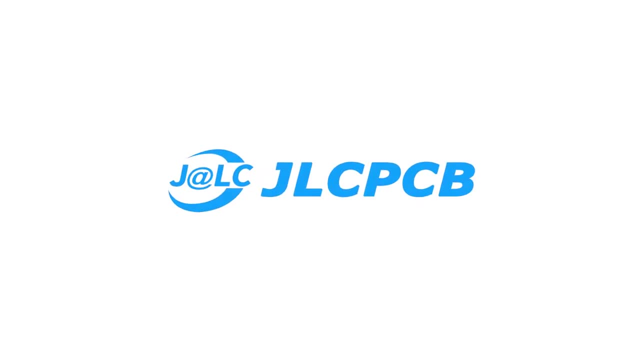 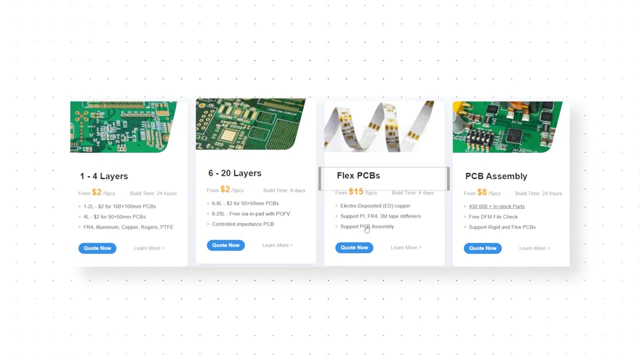 website to place the order. By the way, a big thanks to JLCPCB for sponsoring this video. They are a leading manufacturer of printed circuit boards, offering a wide range of PCBs and top-notch PCB assembly services at affordable prices. Their user-friendly ordering system. 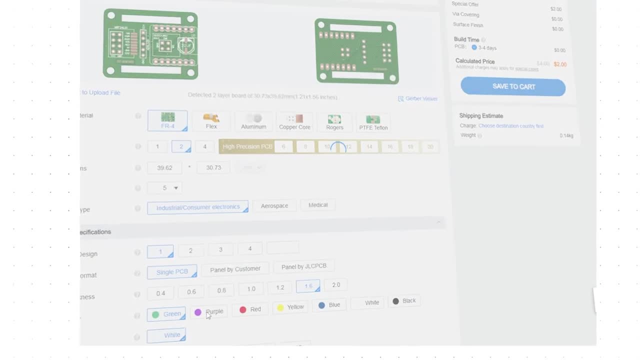 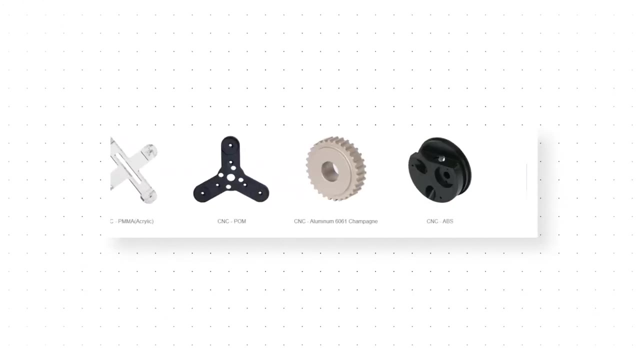 provides instant quotes, making it easy for anyone to order the PCB they need. Plus, JLCPCB also provides 3D printing services with various materials. So let's get started. So if you are ready to take your projects to the next level, head over to JLCPCB using 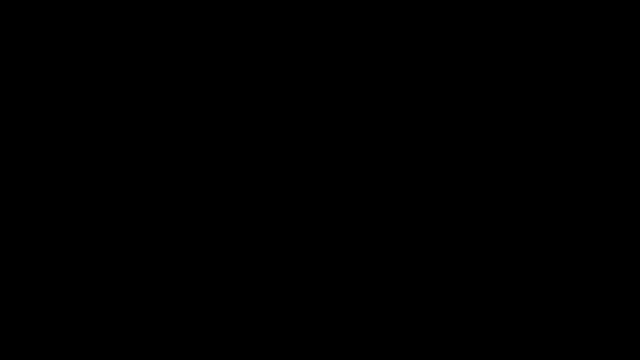 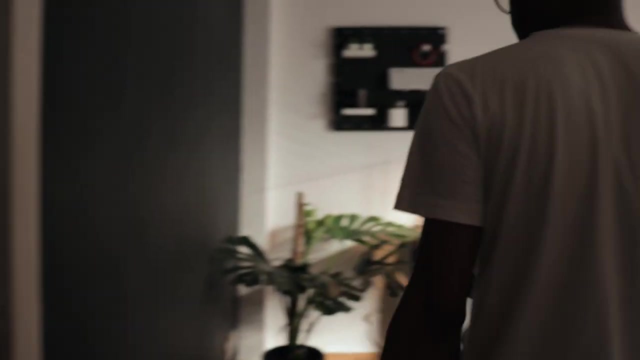 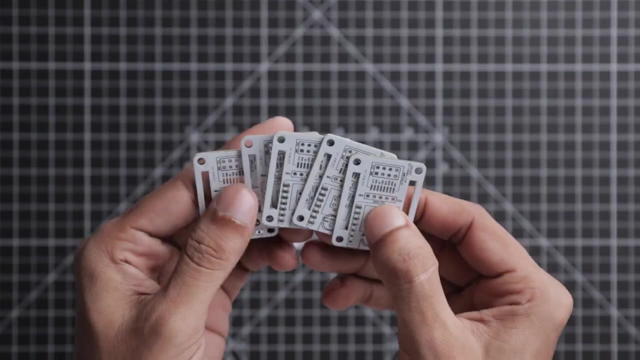 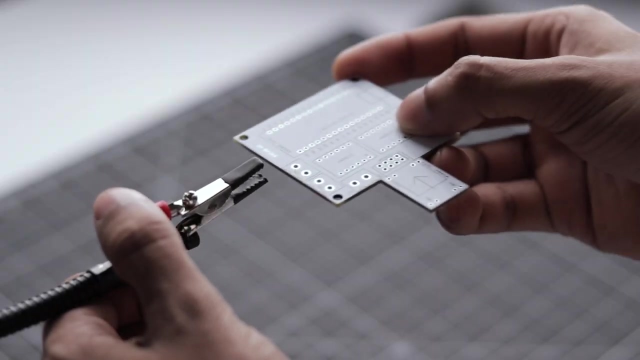 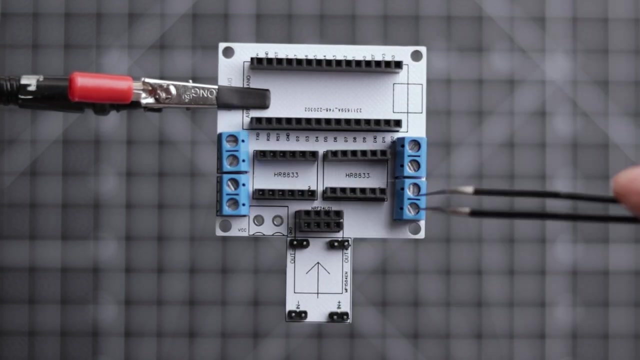 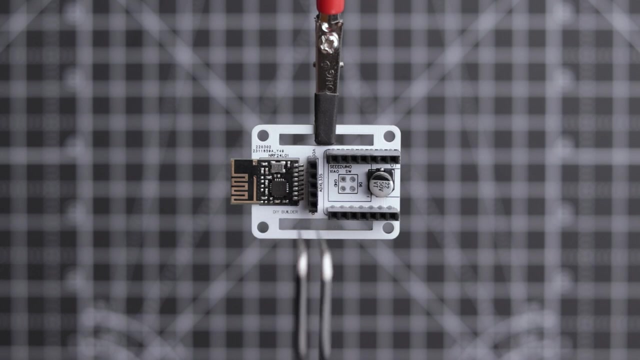 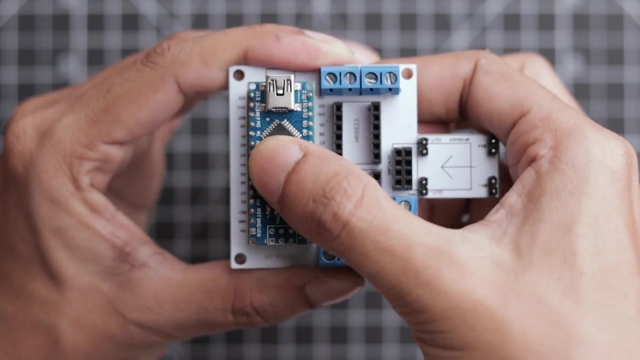 the link in the video description and let them handle the rest. The PCB delivery just arrived and take a look at the quality. These PCBs are absolutely top-notch. Let's quickly solder these header pins and screw terminals. Okay, guys, soldering done. Now it's time to mount the arduino nano h parody motor driver. 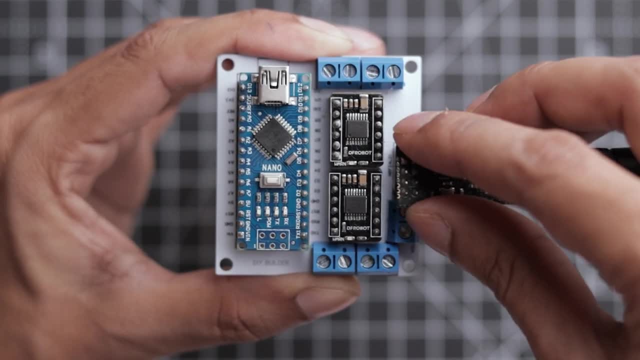 buck converter and nrf24-l01 radio module to this circuit. Now let's mount the Arduino Nano hr8833 motor driver, buck converter and nrf24-l01 radio module to this circuit. This is going to take about 10 minutes and you can make up to 120,000 proudly today. 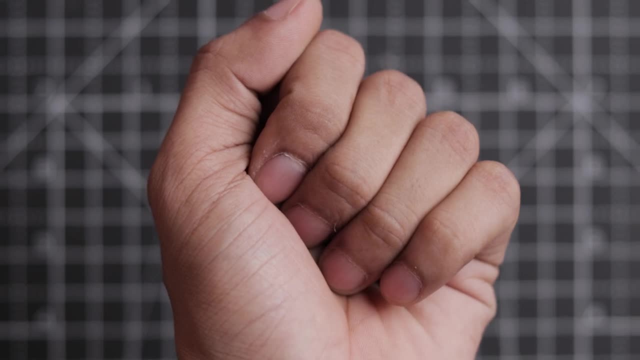 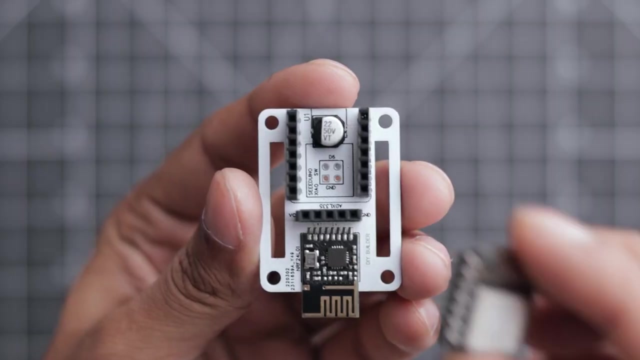 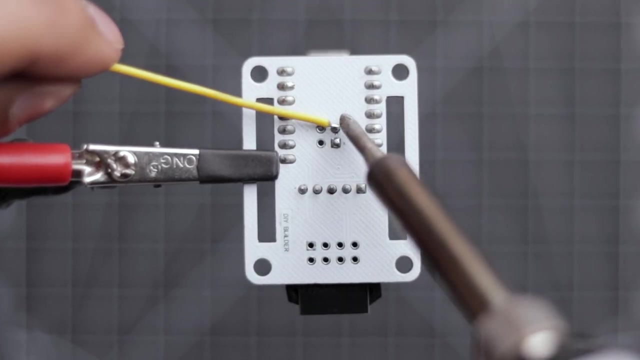 The method of c bus circuit. on the other hand, instead of arduino nano, i'm using the sidvino shower for the transmitter circuit, due to smaller size. okay, let's quickly mount the sidvino shower and adxl 335 accelerometer sensor to the transmitter circuit. finally, let's complete this circuit by sorting. 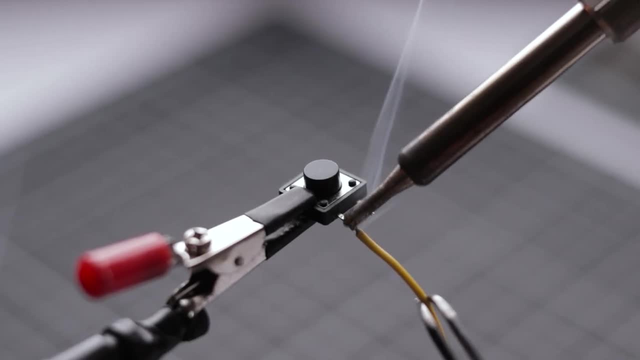 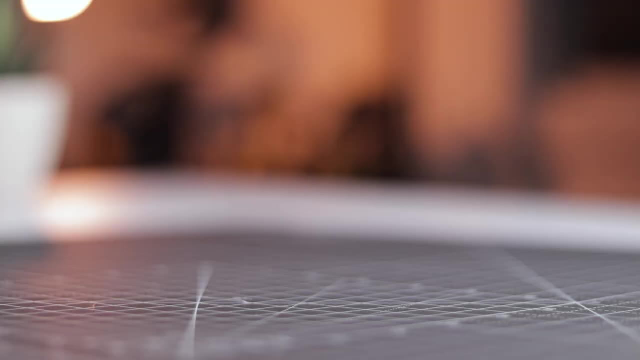 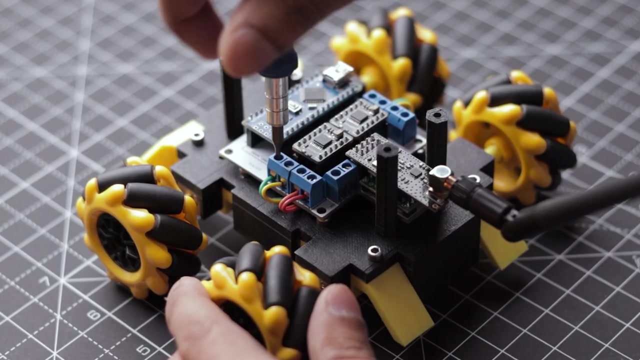 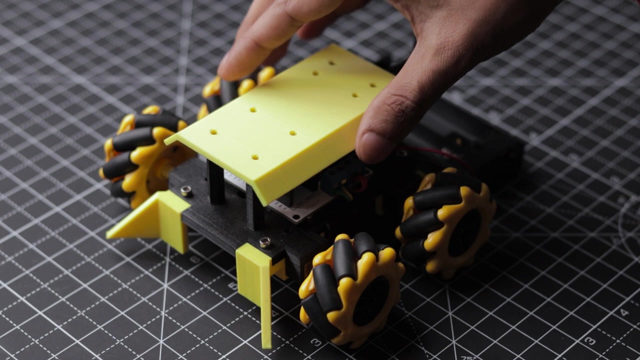 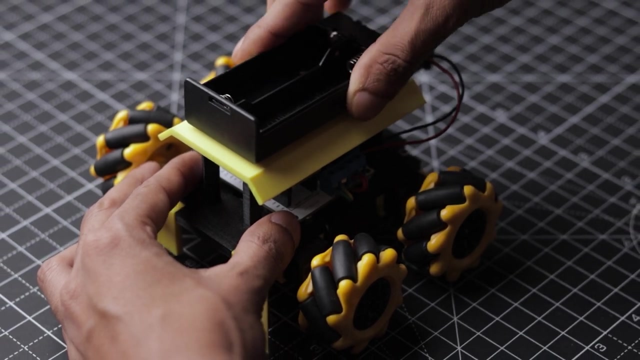 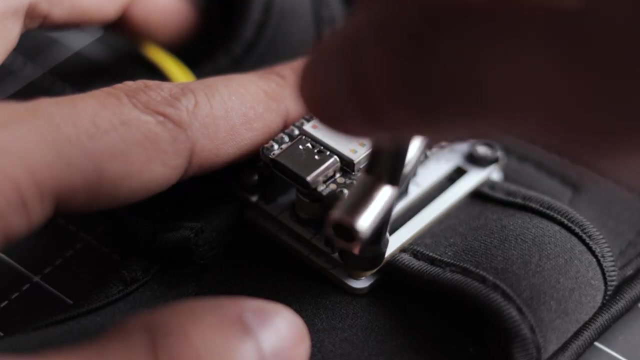 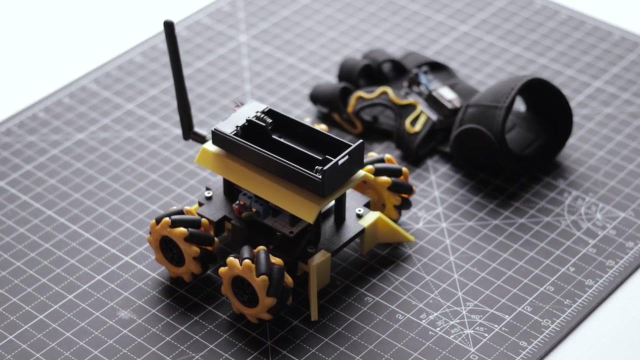 the push button. both circuits are successfully assembled and ready for installation, so let's move forward with the rest of the assembly process. all right, guys, the robot is almost ready. now let's prepare the hand rub great. the assembling part is now complete. it's time to move on to the next step. 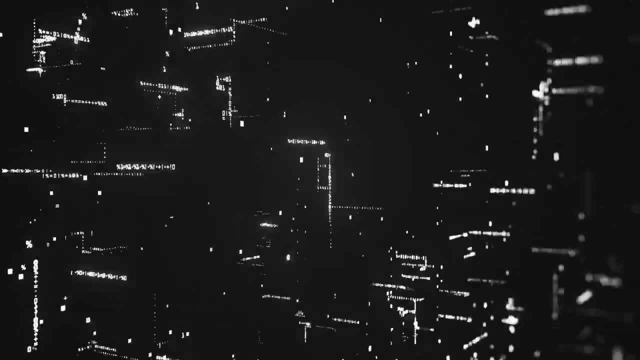 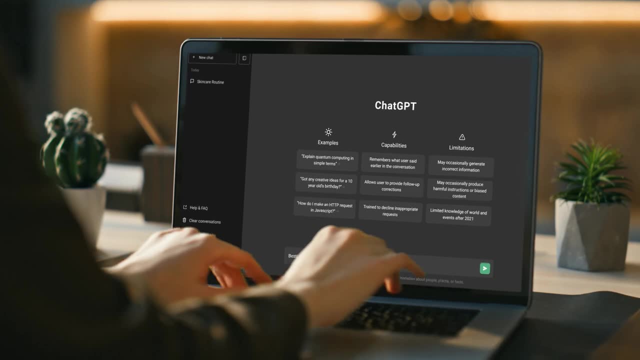 get excited, guys. it's programming time. this is where ai is gonna show its magic. here i'm using chat gpt for this project, which is a powerful ai language model. i guess you already know how it works, so there's no need for further explanation. with that in mind, i asked you to generate the 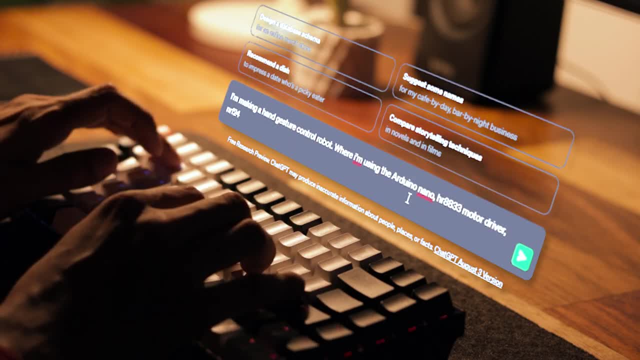 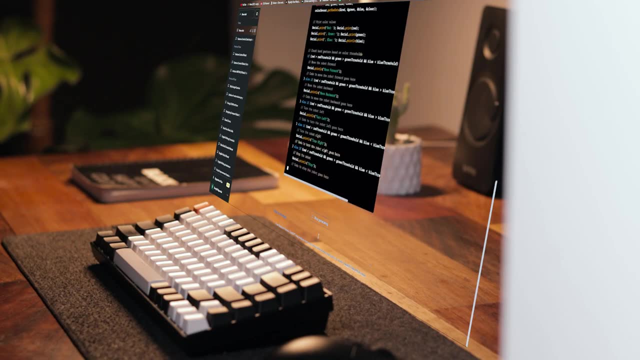 code structure for the transmitter and the receiver circuit. surprisingly, chat gpt generated code for both circuits, which is the same as the transmitter circuit and the receiver circuit, in a few seconds, which is freaking dope. however, it's not a complete code. rather, it's a foundational structure that provides a simple framework for communication and gesture recognition. 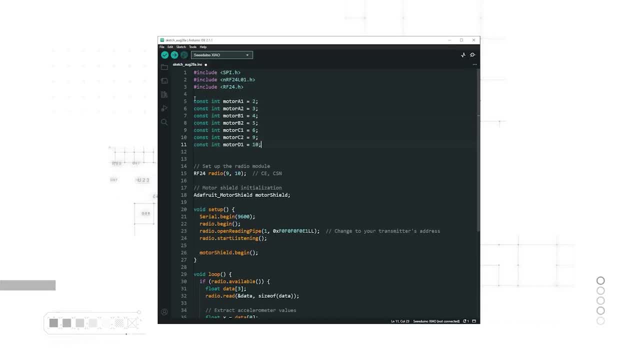 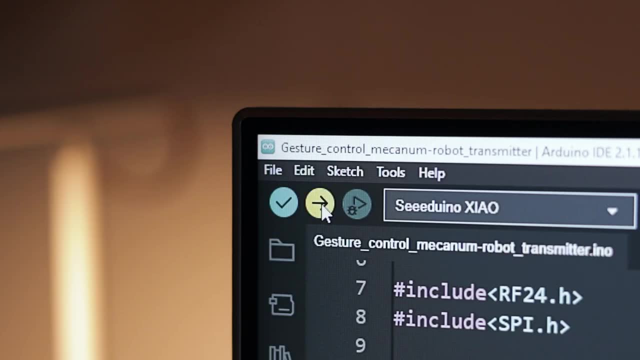 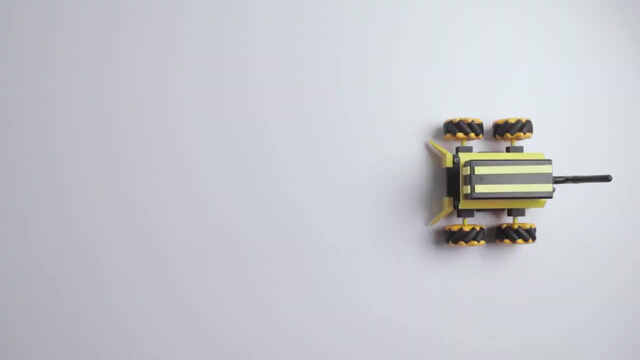 we will need to customize it according to our requirements. all right, i have made a lot of adjustment in the course for this project. now let's quickly upload the codes and check whether the codes are working or not. after uploading the course, i quickly installed the batteries to power up these circuits. okay, both circuits are now powered on. let's see if it works. 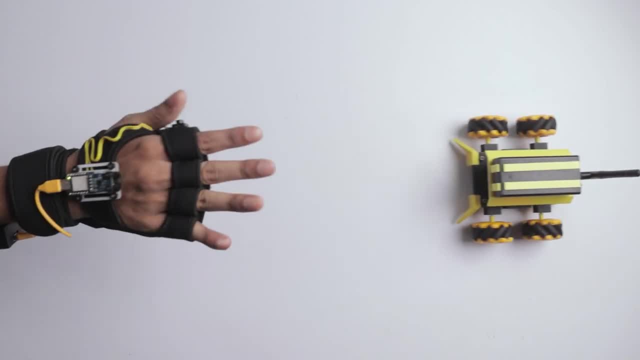 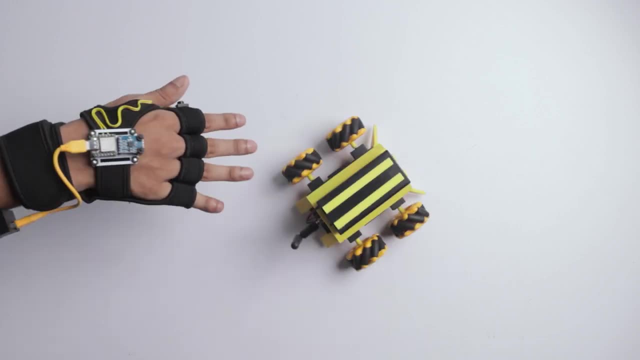 and so i'm gonna go ahead and start the test. the robot is responding to my hand gesture flawlessly, which means the codes are working like a charm, but the robot's movement seems somewhat limited, whereas it's designed to have the freedom to move in any direction. 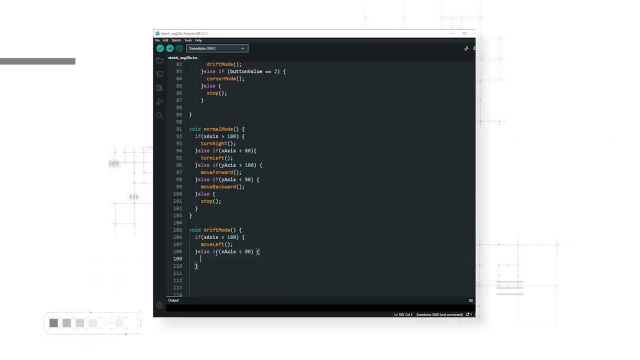 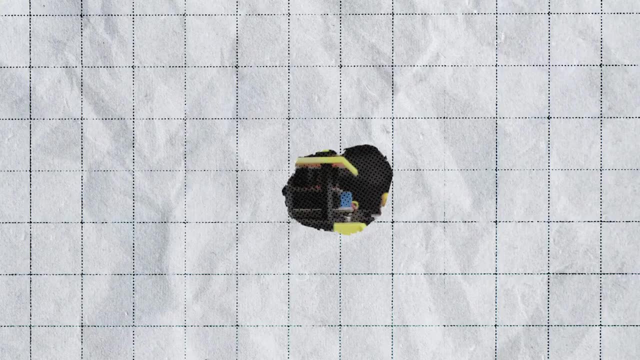 to unlock its full potential. i've added some fresh new commands into the code, then re-uploaded the code again, and here's the final output: a robot that glides in any direction. now let me show you how this robot works well. it features three exciting modes. in normal mode it 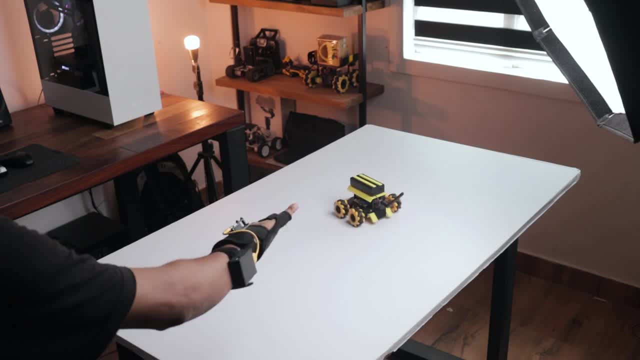 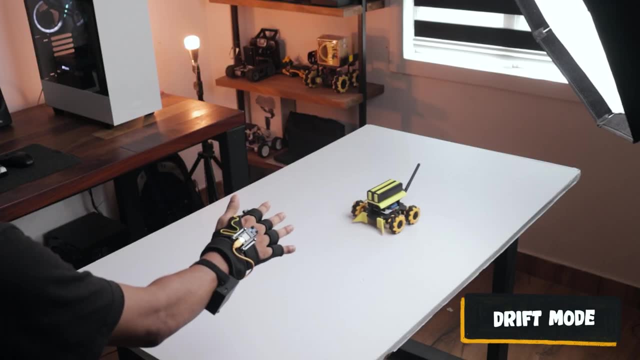 will go forward, backward and left and right according to hand gestures, but when you press the push button, the robot switches to drift mode. in this mode, you have the power to drive this robot sideways. but wait, there's more. if you press the push button one more time, the robot shifts to. 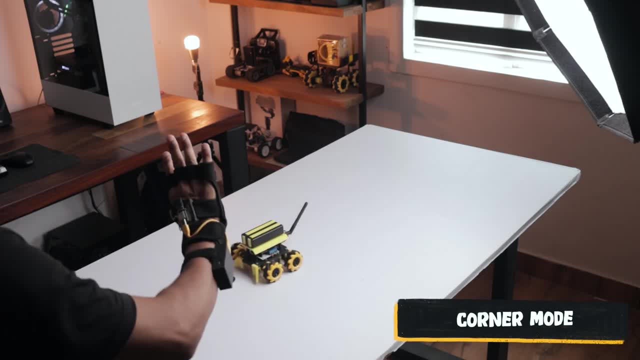 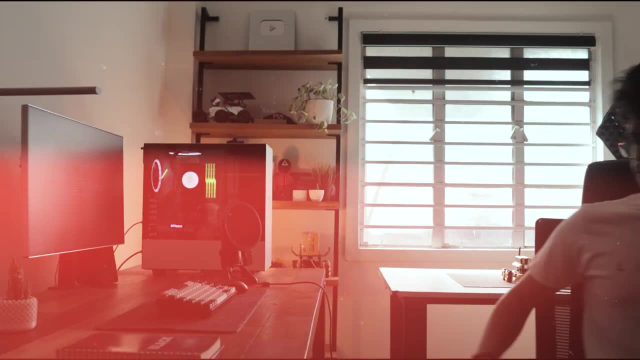 corner right mode. in this mode, the robot skillfully maneuvers toward the corners based on your hand gesture, and that's the magic of this unique robot. so i'm going to show you how this robot works. so i'm going to show you how this robot works. that's it for today's video, and i hope. 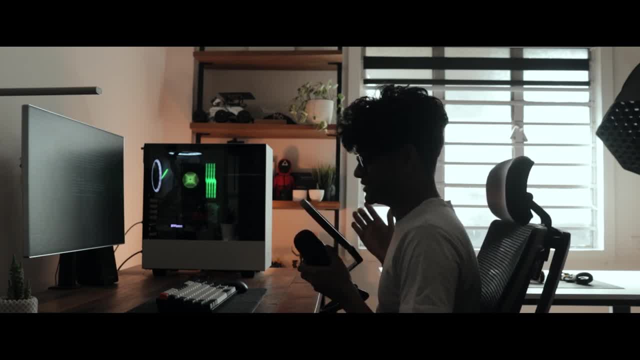 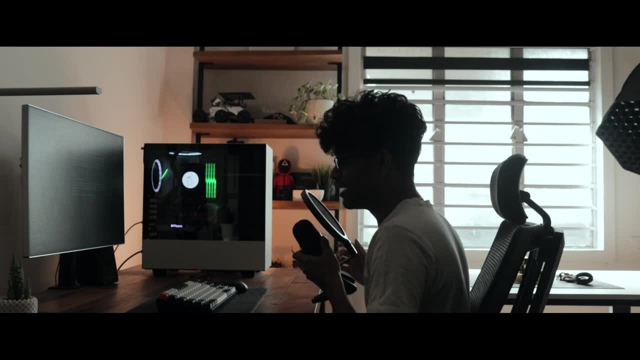 you enjoyed this video. if you did, then make sure to hit that like button. it means a lot to me, and don't forget to subscribe for more awesome future projects. if you have any project ideas, then feel free to share them in the comment down below. i still read and reply to almost every single. 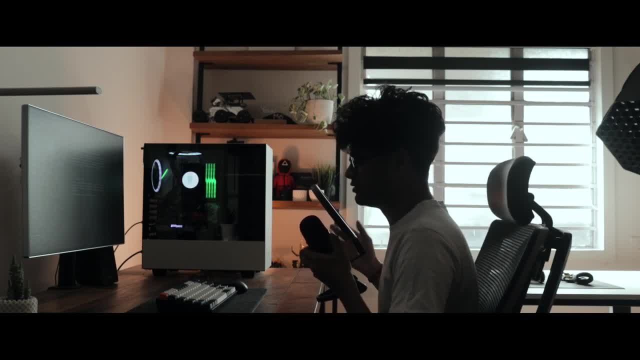 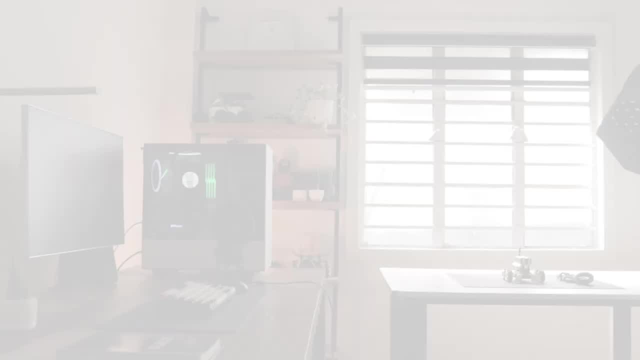 comment. thank you for watching till the end and hopefully see you guys soon. bye.